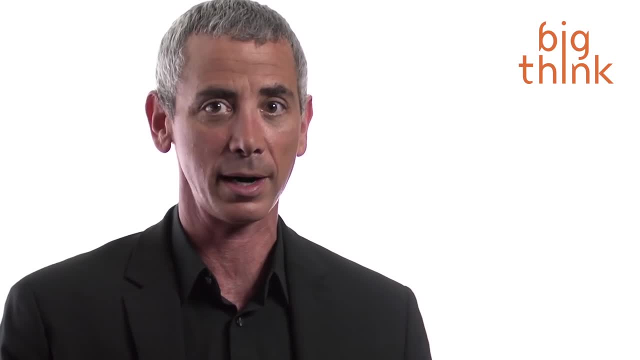 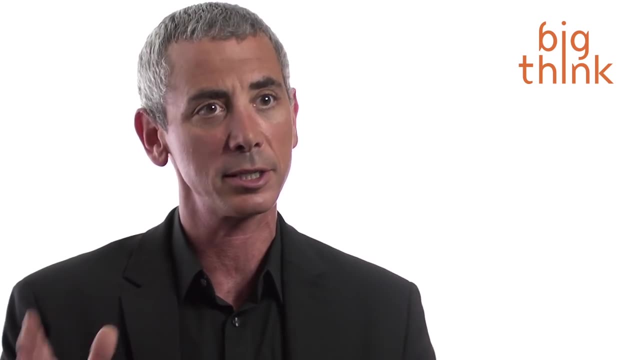 I'm in. So I started looking at it and I just started I said, okay, I'm just going to read. I'm going to go back ten years and read the articles in major journals- New England Journal of Medicine, Science, Nature, that kind of thing, Not even going to go that deep, Very. 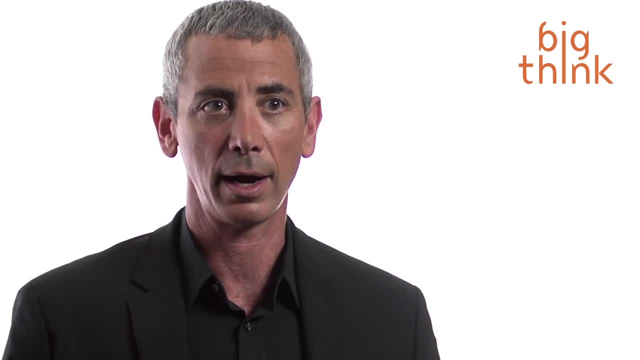 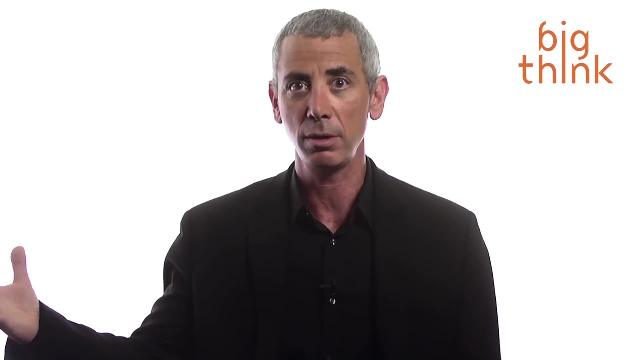 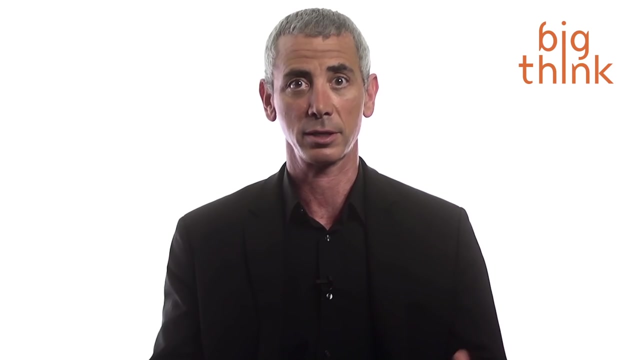 very quickly. what I started to discover is every single thing I thought I knew about steroids. Steroids was wrong. Every crazy disease these drugs had been linked to had nothing to do with it. I'll give you a phenomenal example: Steroids were linked to liver cancer: liver. 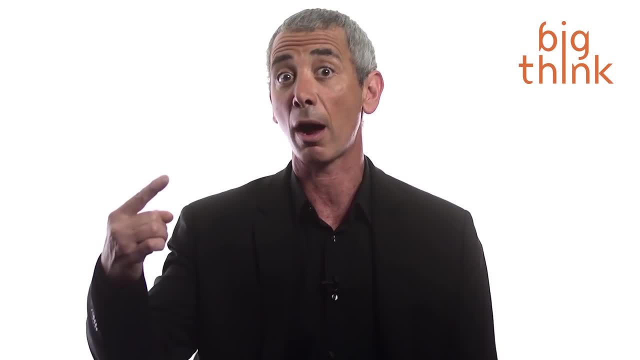 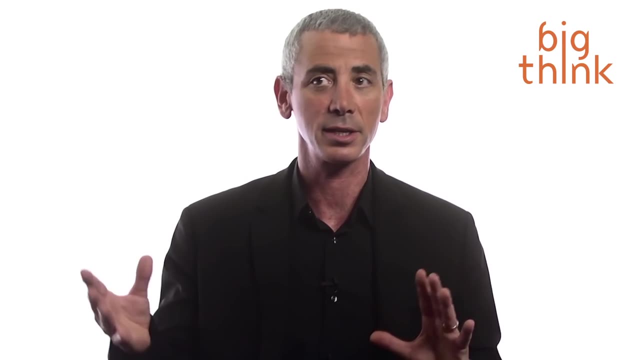 problems right, Nothing to do with the steroid. It has to do with the coating they put around the steroid so it could pass through the stomach and get into your bloodstream. That was what was causing the problems. That coating obviously has since been replaced. But Nick Evans, who's? 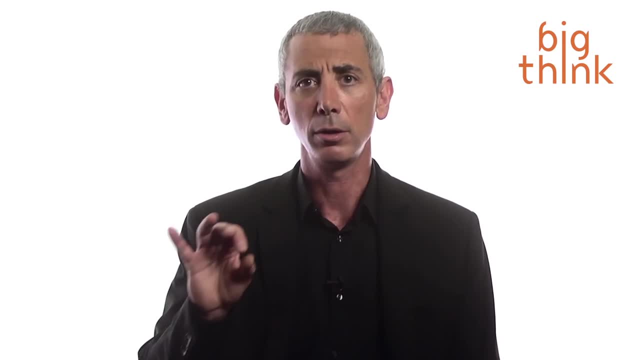 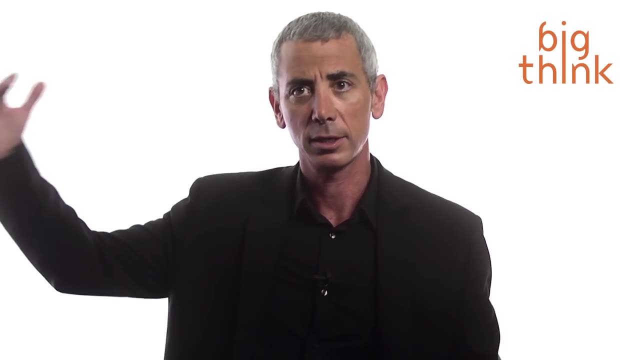 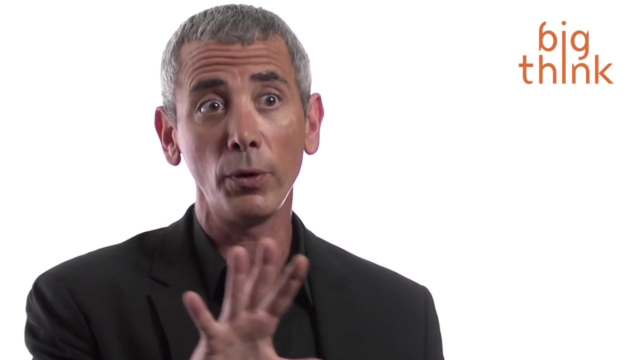 at UCLA is the only person literally in history who has ever done long-term steroid studies right: Long-term abusers, bodybuilders, double and triple, stacking steroids for ten, twenty years at a time. None of the things we've been told about are real. The only danger he found is, since the heart is a muscle, there's. a certain point. if you're taking massive, massive doses over long periods of time, it can expand. It could grow right And grow bigger than the blood vessels and the ventricles and whatnot, which would be a problem. This doesn't mean, by the way, when teenagers use steroids right when you're still producing. 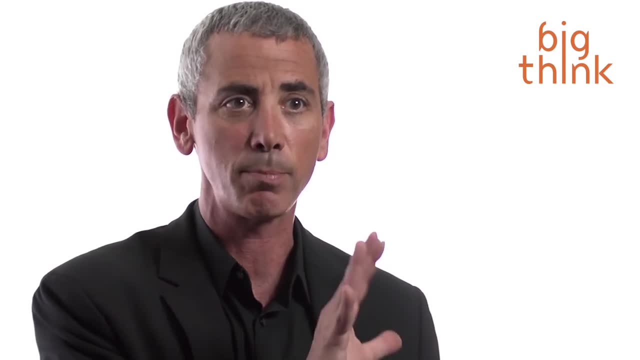 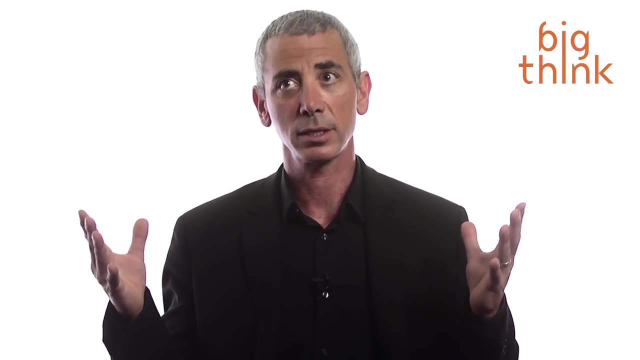 lots of these substances. it's an absolute disaster. right, That's bad news. But in adults, everything we've been told tends to be wrong, And some of what we've been told cost millions of lives. right Turns out, steroids are phenomenal. phenomenal in fighting back AIDS. They're 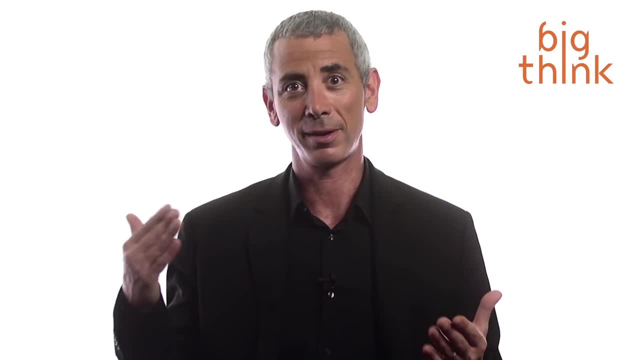 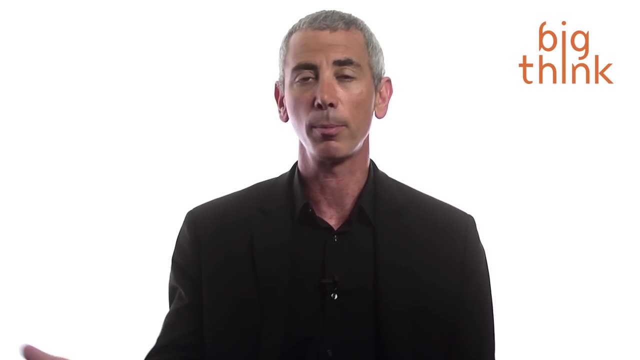 really really, really good. Nobody wanted to talk about it when doctors started treating AIDS patients with it. The guy who started doing this was a guy named Walter Jekoff. The government jumped in and put him in jail for five years. He scared the hell out of a ton of doctors And the 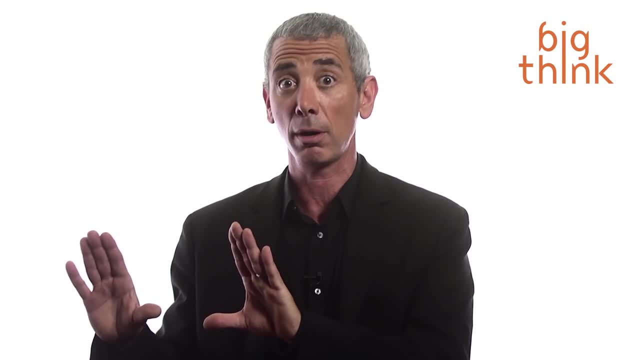 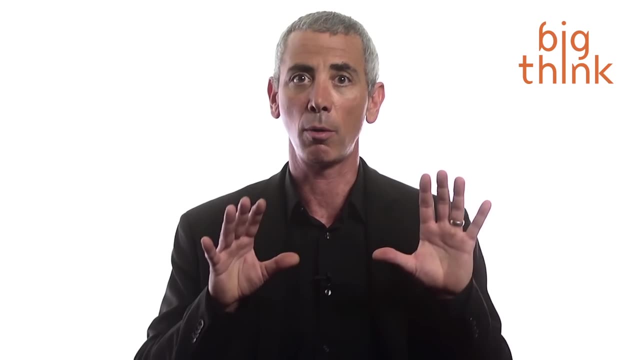 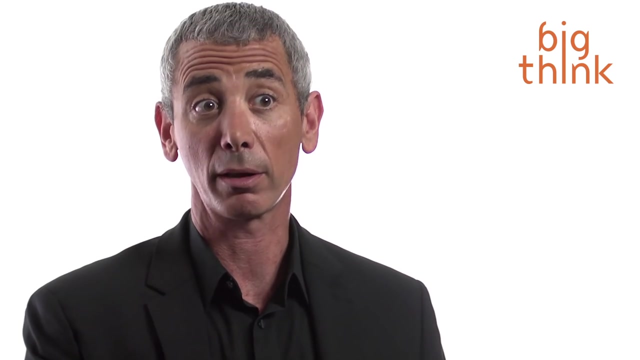 result of this kind of us trying to keep sports pure and, you know, preserve the competitive advantage has been millions of people died as a result. So not only is everything you've been told about steroids wrong, but there were a lot of consequences. The people who 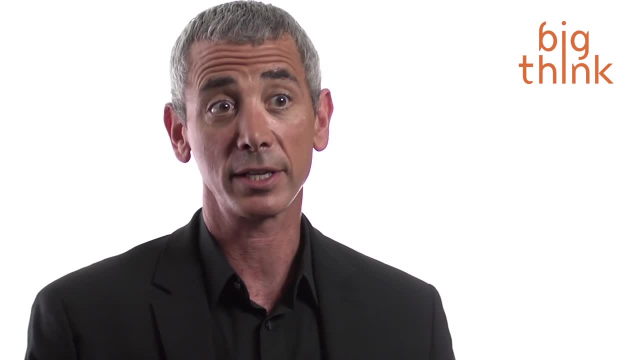 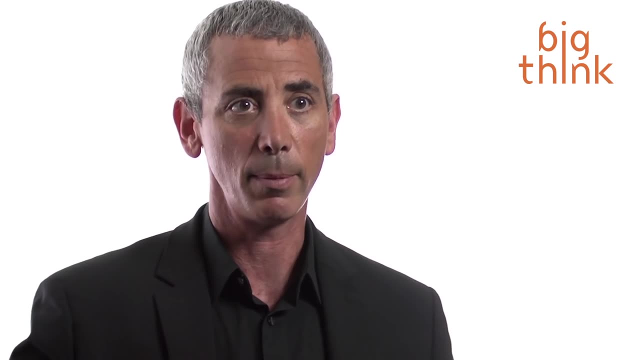 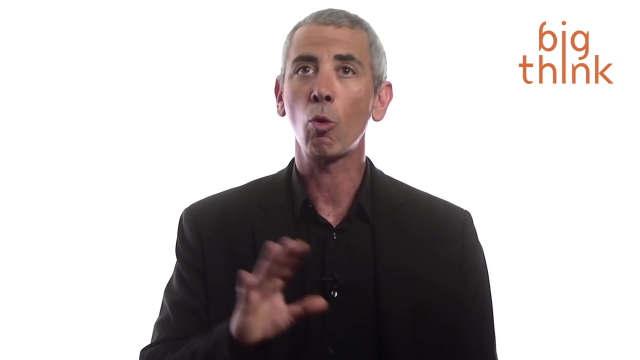 have been at the forefront of this and kind of pushing it forward. is the life extension community right? Our hormones decline as we age, So the idea here is we can replace them, And they've been working on this stuff for 10, 15 years, at this point with some success. It is now one.